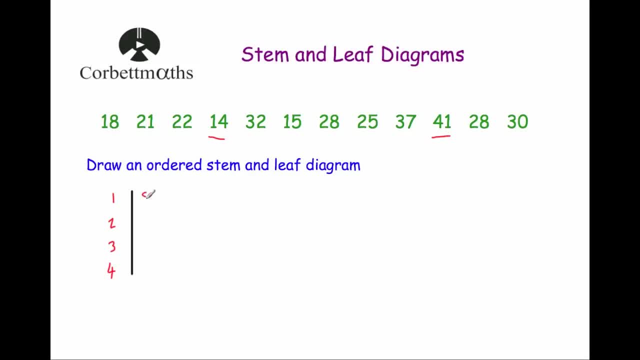 let's do it unordered to begin with. So we've got 18.. So we'll put an 8 here. So that's 18.. We've got 21.. So let's just cross off our 18.. And if you're crossing this off on, 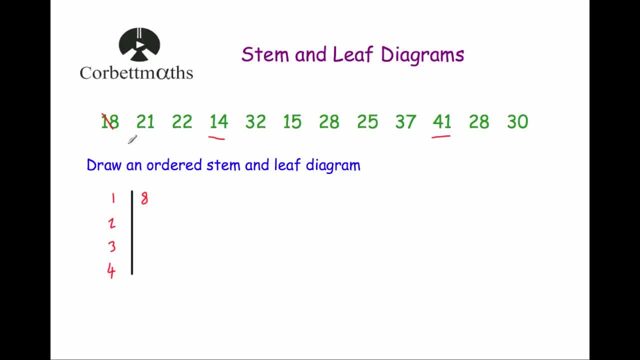 a test or for homework. do it in pencil, just so that you can rub it out and see the number again, if need be. So then 21.. So we're going to put a 1 in the 20s row. We've got 22.. So we'll just put. 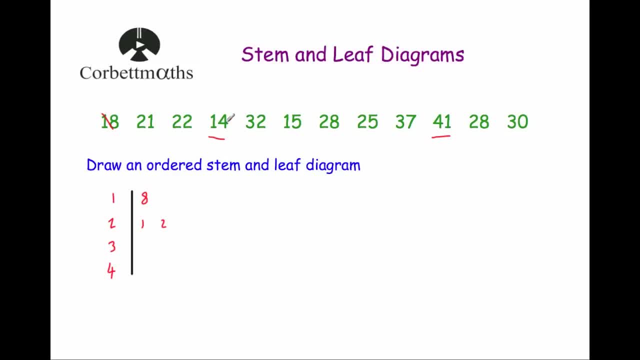 a 2 there and that'll be 21 and then 22.. We've got, and we'll make sure we're crossing off 14.. So we're going to put a 4 in the 10s column, or 10s row A 32. So we're going. 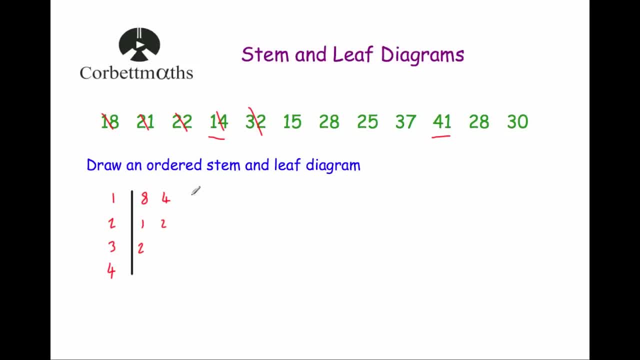 to put a 2 in the 30s row 15.. We'll put a 5 there in the 10s row 28.. So that's an 8 in the 20s row 25.. That's a 5 in the 20s row. 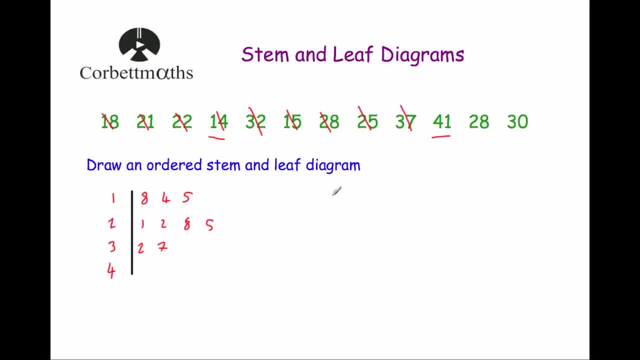 37.. So that's a 7 in the 30s row. 41.. That's a 1 in the 40s row 28.. So that's an 8 in the 20s row And 30. That's going to be a 0 in the 30s row. 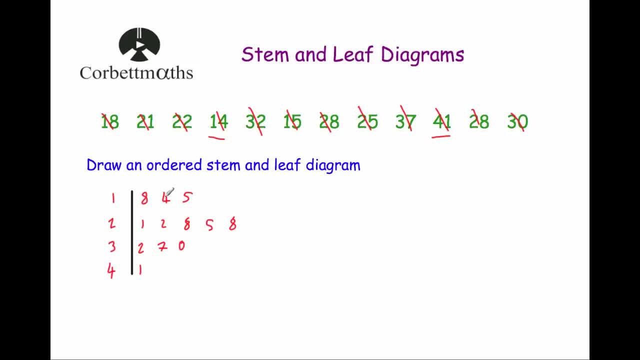 So we've got all our numbers. Let's just check them. So let's count our leaves: 1, 2,, 3,, 4,, 5,, 6,, 7,, 8,, 9,, 10,, 11,, 12.. So let's check our numbers: 1, 2,, 3,, 4,, 5,, 6,, 7,, 8,, 9,, 10,. 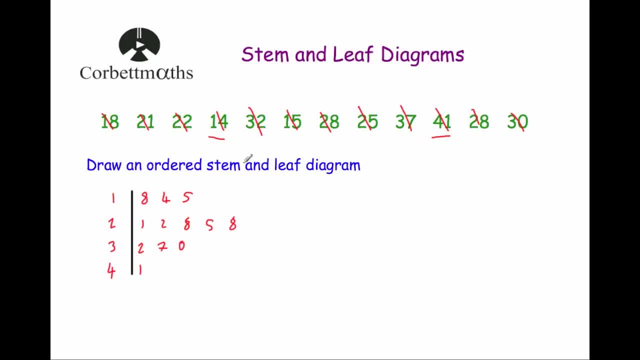 11,, 12.. So we've got all of them, But that's an unordered stem leaf diagram. We were asked we're going to draw an ordered one. So what we're now going to do is we're now going to put them in order. So let's draw our line again like: so We'll put our stems in. So. 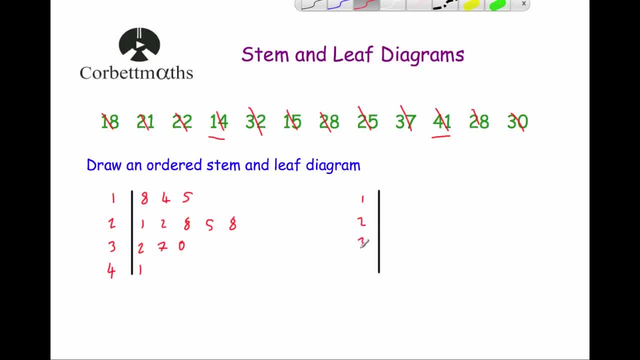 our 10s, 20s, 30s and 40s. And now we're going to put our leaves in order in each row. So we had 18,, 14, and 15.. So we're going to put the 4 first, then the 5, and then the. 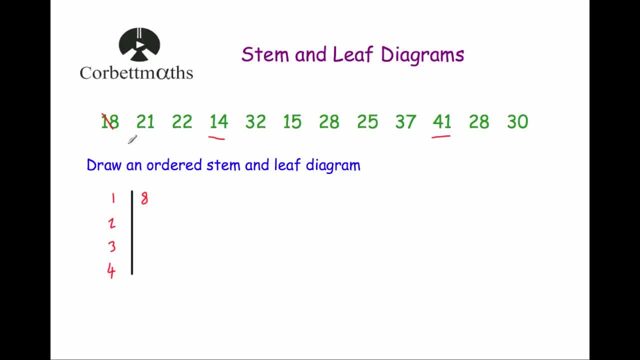 a test or for homework. do it in pencil, just so that you can rub it out and see the number again, if need be. So then 21.. So we're going to put a 1 in the 20s row. We've got 22.. So we'll just put. 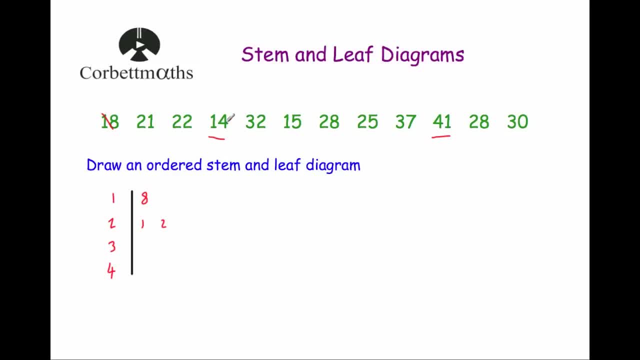 a 2 there and that'll be 21 and then 22.. We've got, and we'll make sure we're crossing off 14.. So we're going to put a 4 in the 10s column, or 10s row A 32. So we're going. 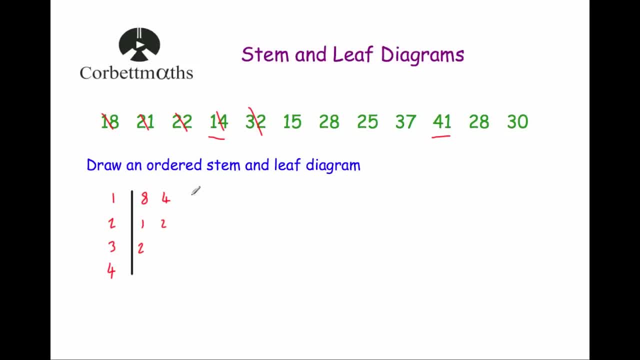 to put a 2 in the 30s row 15.. We'll put a 5 there in the 10s row 28.. So that's an 8 in the 20s row 25.. That's a 5 in the 20s row. 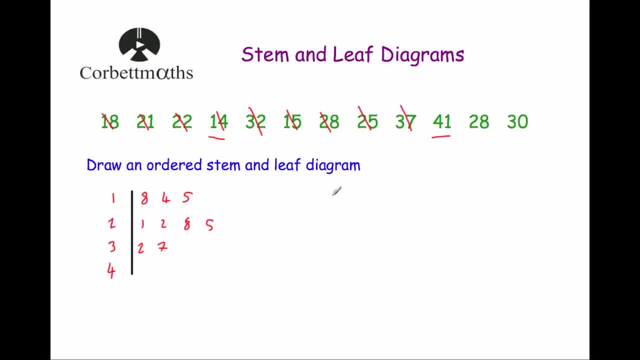 37.. So that's a 7 in the 30s row. 41.. That's a 1 in the 40s row 28.. So that's an 8 in the 20s row And 30. That's going to be a 0 in the 30s row. 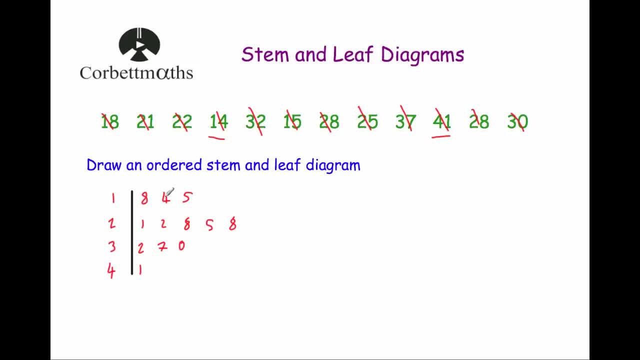 So we've got all our numbers. Let's just check them. So let's count our leaves: 1, 2,, 3,, 4,, 5,, 6,, 7,, 8,, 9,, 10,, 11,, 12.. So let's check our numbers: 1, 2,, 3,, 4,, 5,, 6,, 7,, 8,, 9,, 10,. 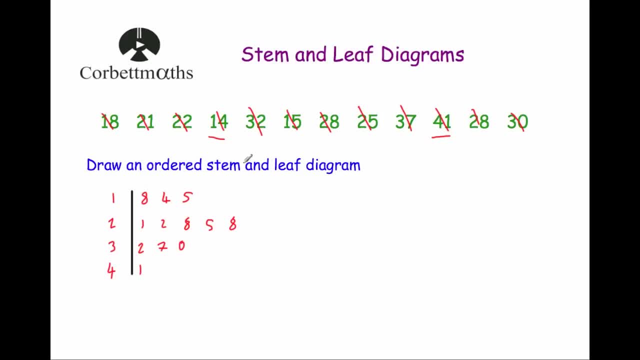 11,, 12.. So we've got all of them, But that's an unordered stem leaf diagram. We were asked we're going to draw an ordered one. So what we're now going to do is we're now going to put them in order. So let's draw our line again, Like: so We'll put our stems in. So 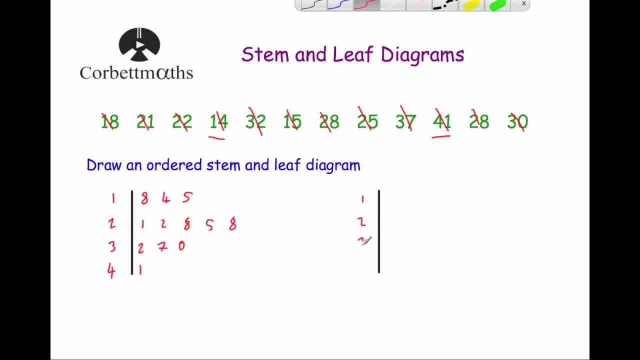 our 10s, 20s, 30s and 40s. And now we're going to put our leaves in order in each row. So we had 18,, 14, and 15.. So we're going to put the 4 first, then the 5, and then the. 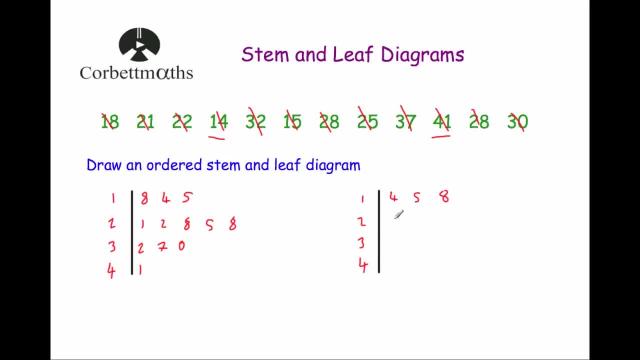 8.. Now we're going on to our 20s row. We're going to put our 1,, then the 2,, then the 5, and then our 2e, Our 8s, Our 30s row. we're going to put our 0 for 30, and then 32, and then the 7 for 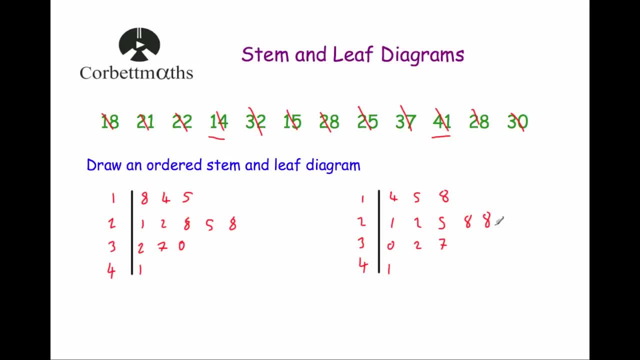 37, and then 41. So we're almost done. We've got our ordered stem and leaf. Now we just need a key. So we're going to write a key, And a key just tells the person who's looking at it how to read it. We know already that this is 14,, 15,, 18,, 21,, 22,, 25,, 28,, 28,, 30,. 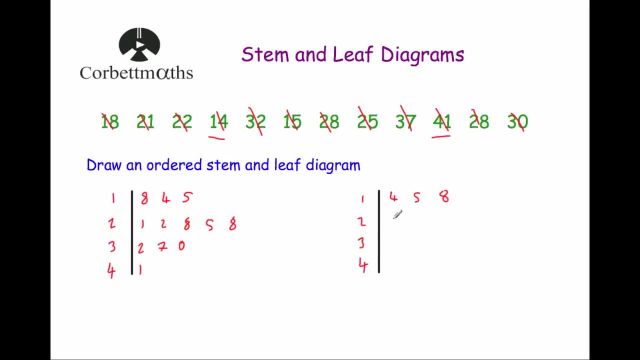 8.. Now we're going on to our 20s row. We're going to put our 1,, then the 2,, then the 5, and then our 2e, Our 8s, Our 30s row. we're going to put our 0 for 30, and then 32, and then the 7 for 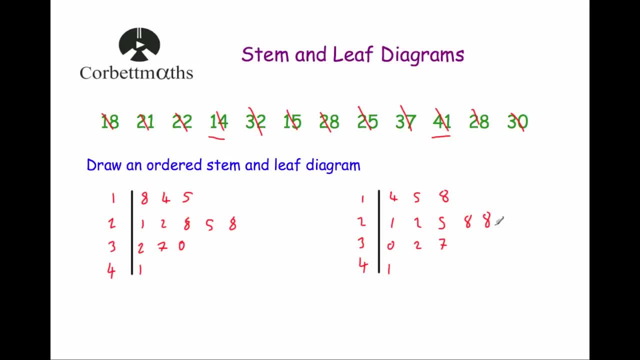 37, and then 41. So we're almost done. We've got our ordered stem and leaf. Now we just need a key. So we're going to write a key, And a key just tells the person who's looking at it how to read it. We know already that this is 14,, 15,, 18,, 21,, 22,, 25,, 28,, 28,, 30,. 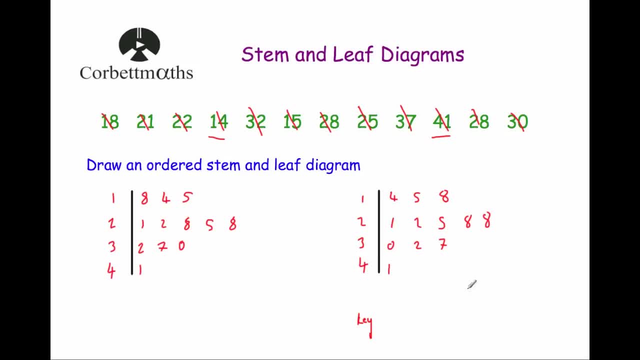 32,, 37, and 41, because we've obviously drawn the stem and leaf diagram, But somebody who's looking at it they're going to be able to read it, So we're going to put our 0 for this Might not necessarily know that these are, that our stem was representing the 10s. 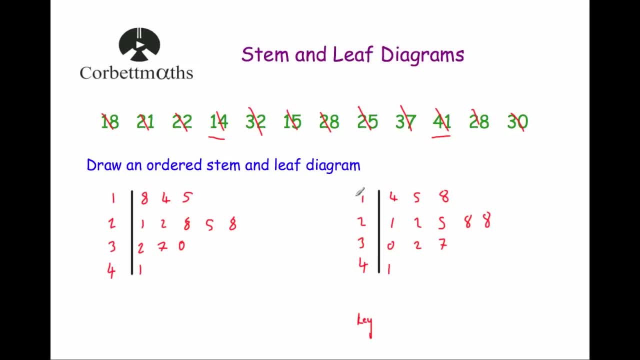 So we need to tell them that. So what we're going to do is I tend to pick the first number, which is 14, and I write 1, and then the line, and then 4 means 14.. So then they know okay. 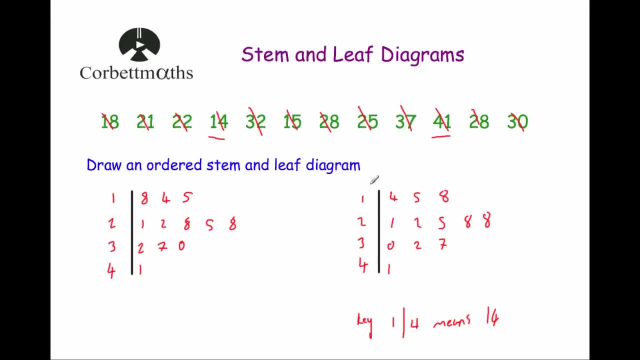 1, line 4 means 14.. So then they can figure out: well, that's going to be 15,, that's going to be 18, and so on. So that is our ordered stem and leaf diagram. All right, so let's have a look at another one. This time I've chosen larger numbers. 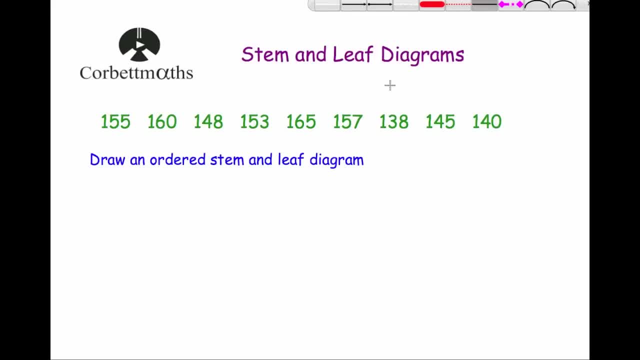 I've chosen numbers in the hundreds, and what we're going to do is we're going to do a stem like so, and we're going to do our own order stem leaf diagram for this, and then our ordered one afterwards over here now with our stem. what we're going to do is we're going to put our hundreds and our tens. 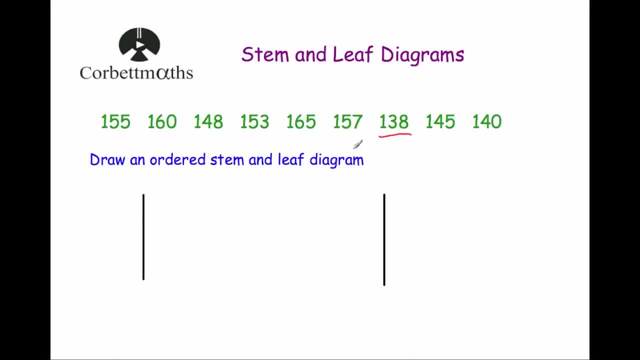 so let's look at our numbers. the smallest number is 138 and our largest number is 165. our numbers are 155, 160, 148, 153, 165, the largest one 157,, 138, 145 and 140.. So we're going from the 130s. 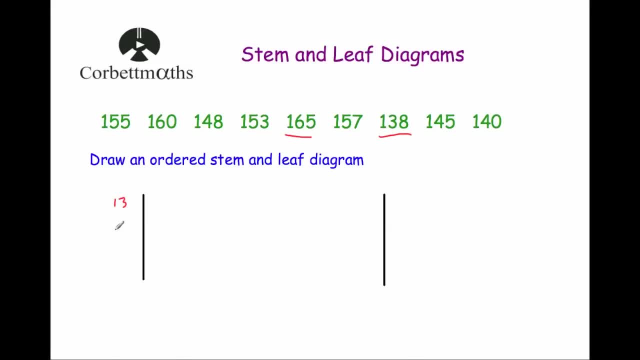 to the 160s. So we're going to put down 130,, 140,, 150 and 160.. And so we'll do that, for we'll do our unordered one, and then we'll do our ordered one over here. So our unordered one to begin with. 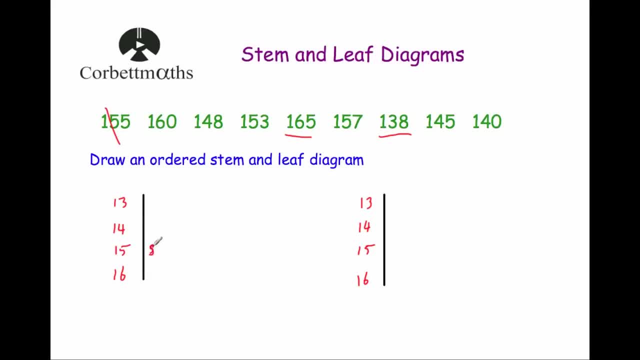 we've got 155, So we'll put a 5 in the 150s row. We'll put a 0 in the 160s row for 160.. An 8 in the 140s row for 148.. A 3 in the 150s row for 153.. 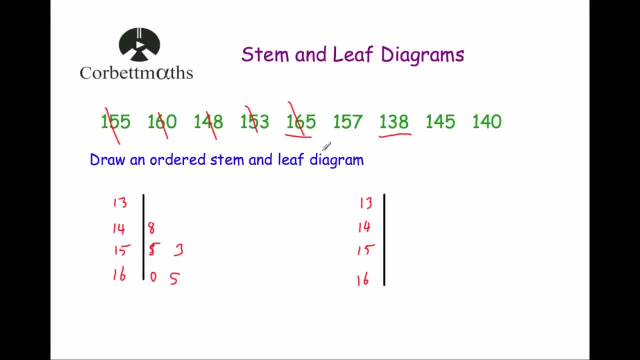 A 5 in the 160s row for 165.. A 7 in the 150s row for 157.. An 8 in the 130s row for 138.. A 5 in the 140s row for 145.. 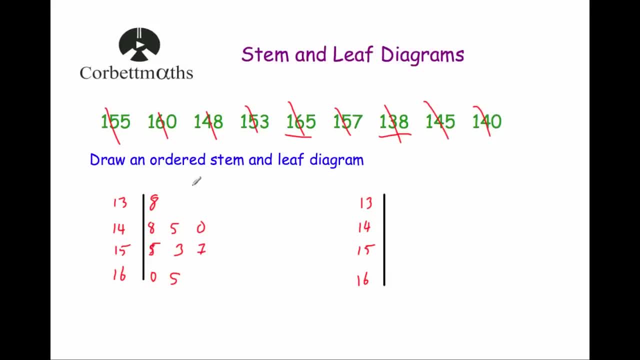 And a 0 in the 140s row for 140.. So let's just count them: 1,, 2,, 3,, 4,, 5,, 6,, 7,, 8,, 9.. So we had 9 numbers. 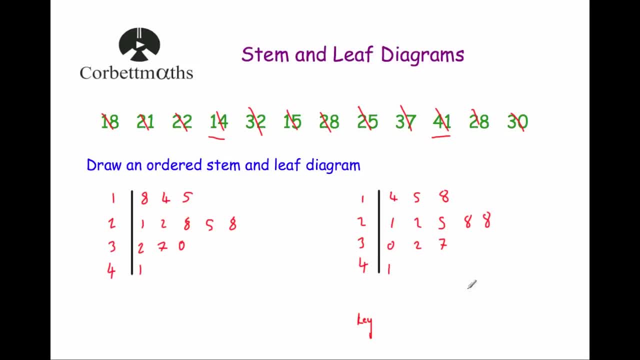 32,, 37, and 41. Because we've obviously drawn the stem and leaf diagram, But somebody who's looking at this might not necessarily know that our stem was representing the 10s, So we need to tell them that. So what we're going to do is I tend to pick the first number, which is 14., And I write: 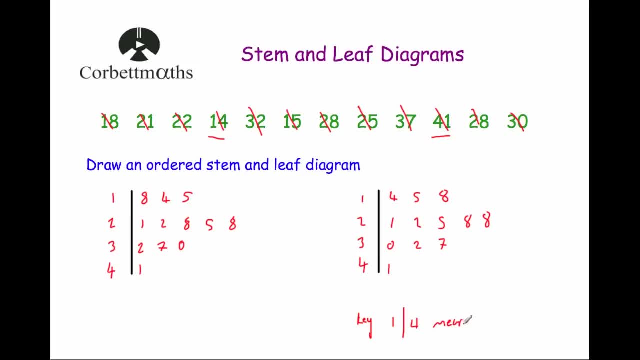 1, and then the line, and then 4 means 14.. So then they know: OK, 1,, line, 4 means 14.. So then they can figure out: well, that's going to be 15,, that's going to be 18, and 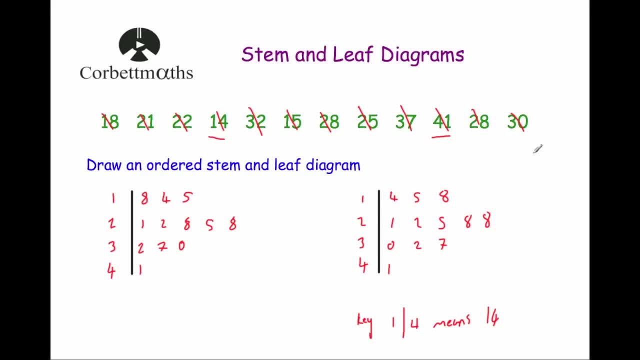 so on. So that is our ordered stem and leaf diagram. All right, So let's have a look at another one. This time I've chosen larger numbers, I've chosen numbers in the hundreds, And what we're going to do is we're going to do a stem like so, And we're going to do 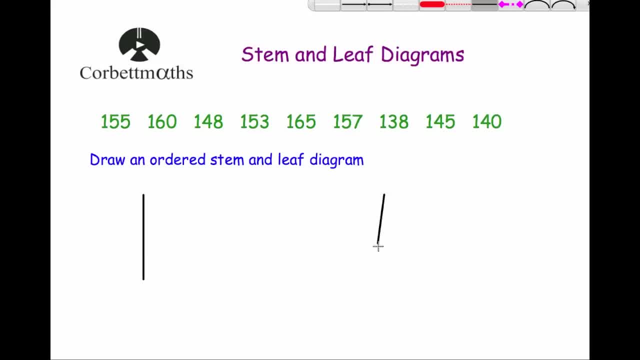 our own ordered stem and leaf diagram for this, and then our ordered one afterwards, over here Now with our stem. what we're going to do is we're going to put our hundreds and our 10s. So let's look at our numbers. The smallest number is 138.. And our largest number is 165. 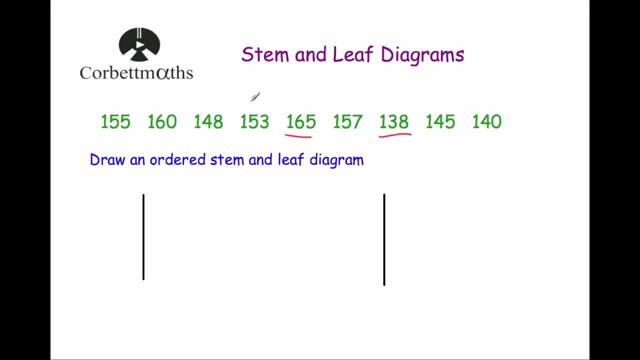 Our numbers are 155,, 160,, 148,, 153,, 165,- the largest one- 157,, 138,, 149, and 150.. So we're going from the 130s to the 160s. So we're going to put down 130,, 140,, 150, and 160. 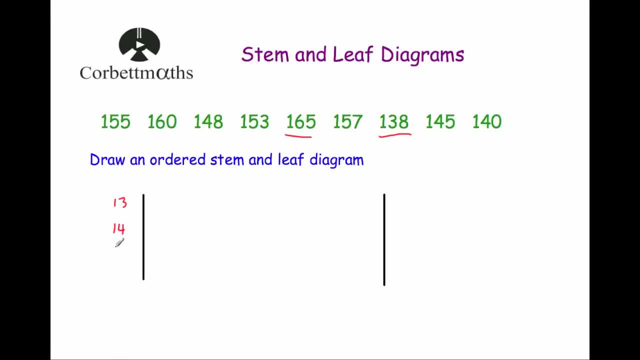 And so we'll do that, for we'll do our unordered one, and then we'll do our ordered one over here. So our unordered one to begin with. So we've got 155.. So we'll put a five in the 150s row. 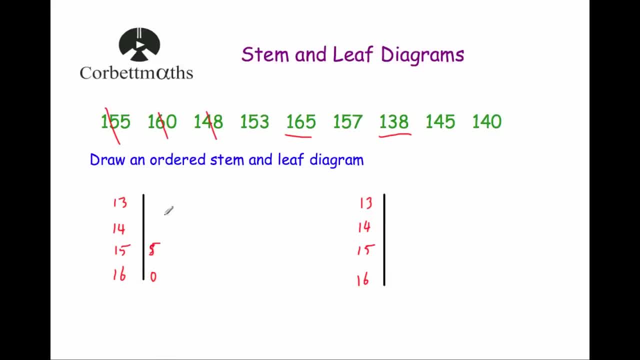 We'll put a zero in the 160s row for 160. And eight in the 140s row for 148.. And then we'll put in a $4.25.. So that's $5.25.. For the $1.75, we take that This is $1.75.. So 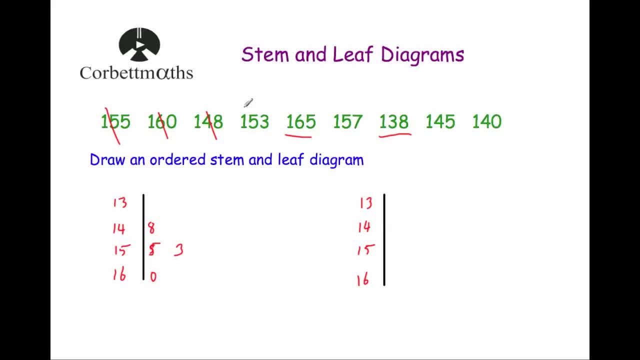 a 3 in the 150s row for 153,, a 5 in the 160s row for 165,, a 7 in the 150s row for 157,, an 8 in the 130s row for 138,, a 5 in the 140s row for 145, and a 0 in the 140s row for 140..